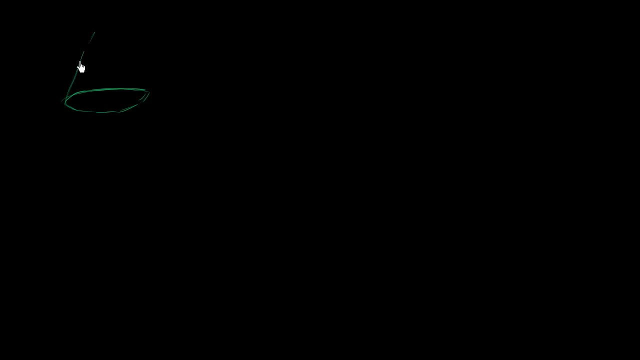 and then it would come to some point, So it would look something like that: This: you could consider this to be a cone, just like that. Or you can make it upside down, if you're thinking of an ice cream cone, So it might look something like that: 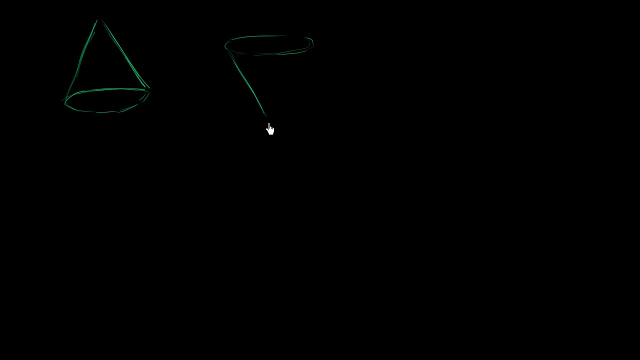 That's the top of it And then it comes down like this: This also is kind of those disposable cups of water you might see at some water coolers And the important things that we need to think about when we want to know about the volume of a cone. 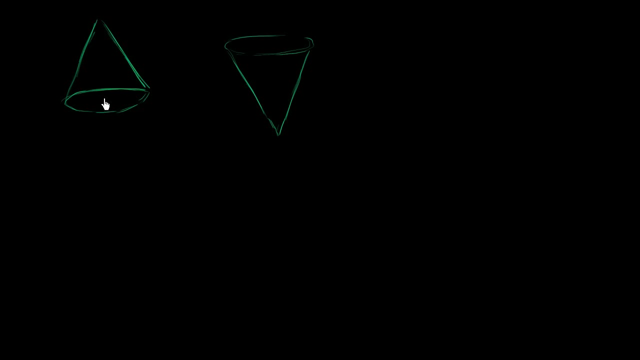 is. we definitely want to know the radius of the base. So that's the radius of the base, Or here's the radius of the top part. You definitely want to know that radius. And you want to know the height of the cone. You want to know the height of the cone. 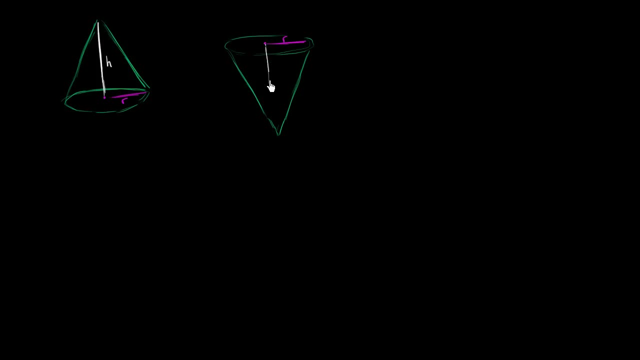 So let's call that h, Or right over here, you could call this distance, right over here, h. And the formula for the volume of a cone, and it's interesting because it's close to the formula for the volume of a cylinder in a very clean way, which is somewhat surprising. 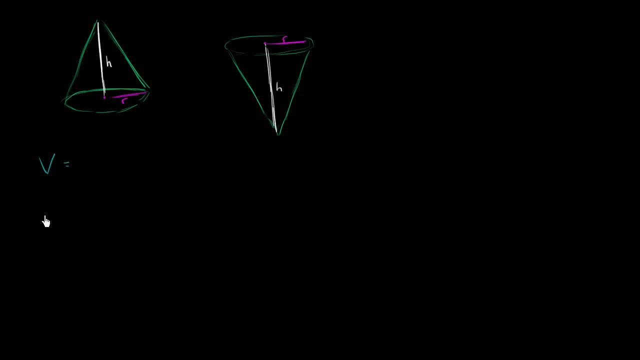 And that's what's neat about a lot of this three-dimensional geometry is that it's not as messy as you would think it would be. It is the area of the base. Well, what's the area of the base? Well, the area of the base is going. 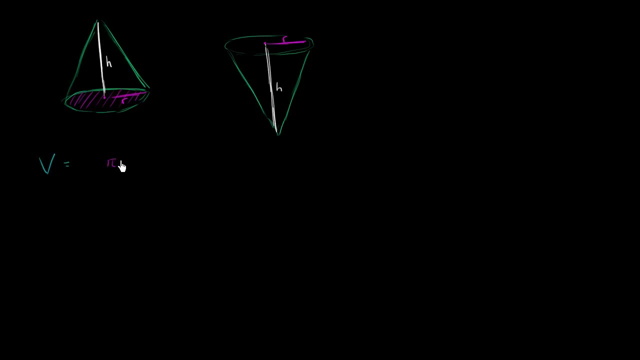 to be pi r squared times the height, And if you just multiply the height times pi r squared, that would give you the volume of an entire cylinder that looks something like that. So this would give you this entire volume that looks of the figure that looks like this: 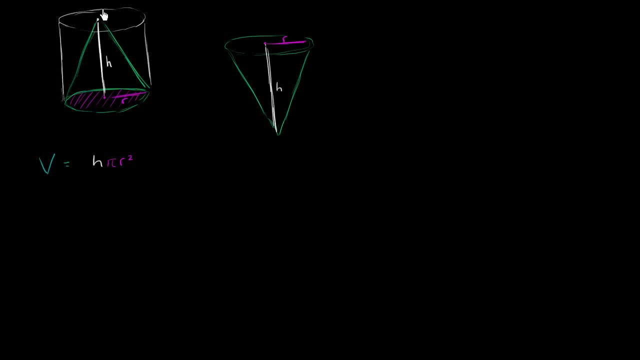 where its center of the top is the top, It's the tip right over here. So if I just left it as pi r squared, h or h times pi r squared, it's the volume of this entire can, this entire cylinder, But if you just want the cone, it's 1 third of that. 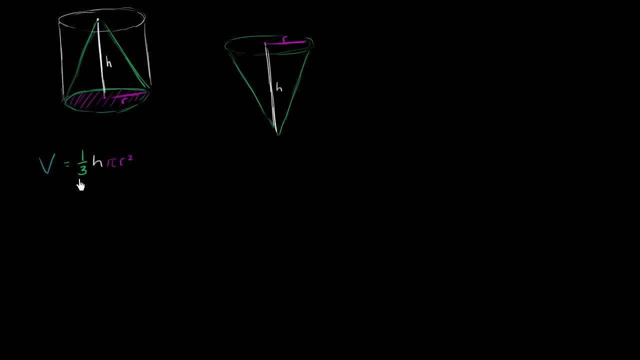 It is 1 third of that And that's what I mean when I say it's surprisingly clean that this cone right over here is 1 third the volume of this cylinder. that is essentially. you could kind of think of this cylinder as bounding around it. 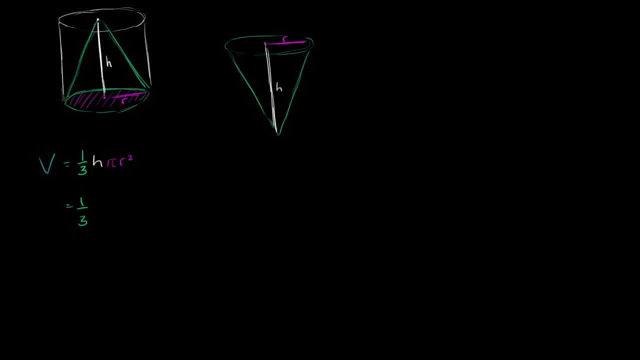 Or, if you wanted to rewrite this, you could write this as 1 third times times pi or pi over 3 times h r squared, however you want to view it The easy way I remember it. for me, the volume of a cylinder is very intuitive. 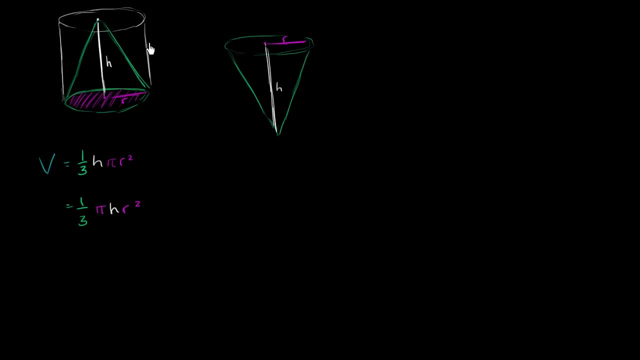 You take the area of the base and then you multiply that times the height, And so the volume of a cone is just 1 third of that. It's just 1 third. the volume of the bounding cylinder is one way to think about it. 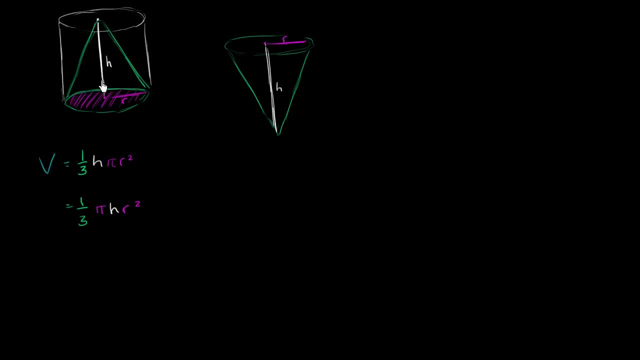 But let's just apply these numbers just to make sure that it makes sense to us. So let's say that this is some type of a conical glass, the type that you might see at the water cooler, And let's say that we're told that it holds. 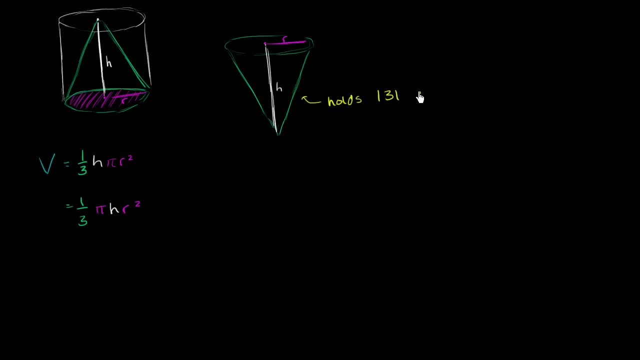 so this thing holds 131 cubic centimeters of water, And let's say that we're also told that its height right over here, which I want to do that in a different color- we're told that the height of this cone is 5 centimeters. 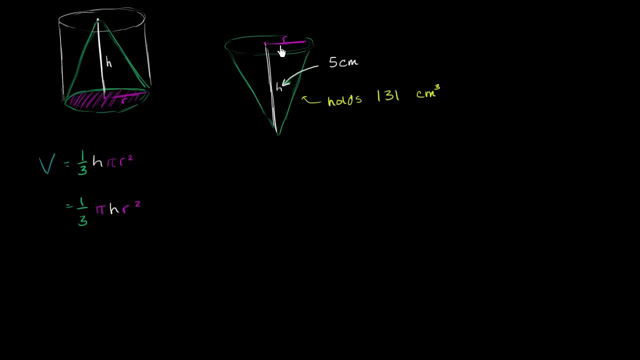 And so, given that if what is wrong, it's roughly the radius of the top of this glass, Let's just say to the nearest tenth of a centimeter, Well, we just once again have to apply the formula The volume, which is 131 cubic centimeters. 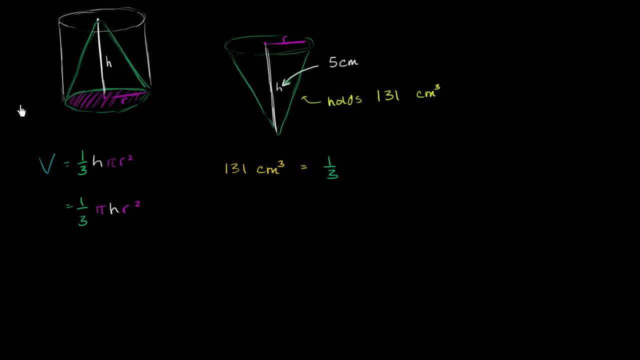 is going to be equal to 1 third times pi, times the height, which is 5 centimeters times the radius squared. If we wanted to solve for the radius squared, we could just divide both sides by all of this business And we would get. radius squared is equal to 131 cubic centimeters. 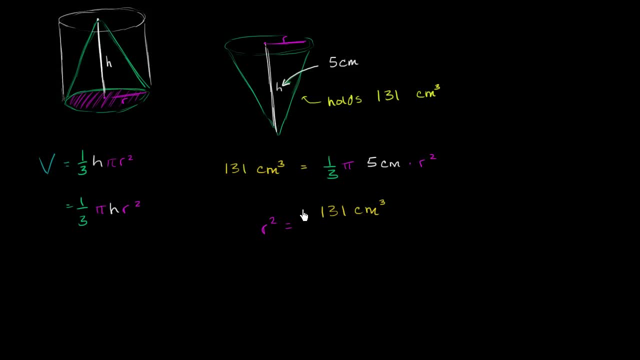 I should say: You divide by 1 third. That's the same thing as multiplying by 3.. And then, of course, you're going to divide by pi And you're going to divide by 5 centimeters. Now let's see if we can clean this up. 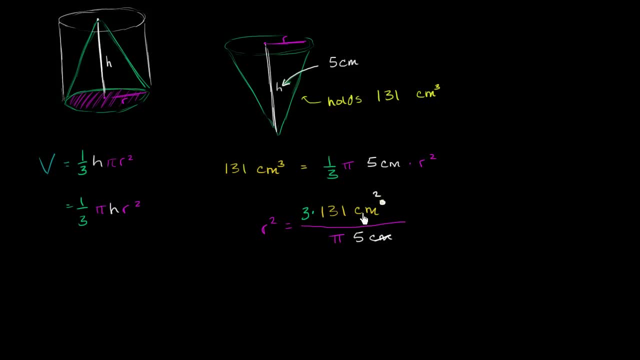 Centimeters, we'll cancel out with one of these centimeters, So you'll just be left with square centimeters only in the numerator, And so this is going to be. and then to solve for r, we could take the square root of both sides.